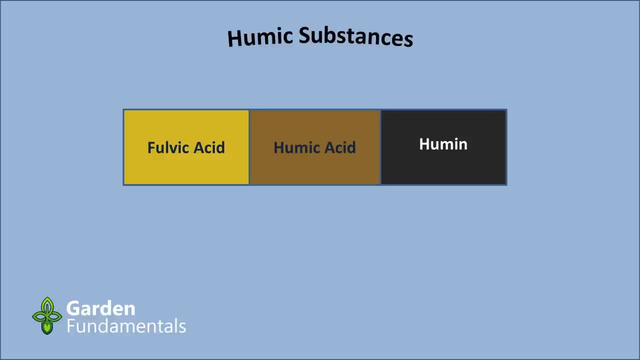 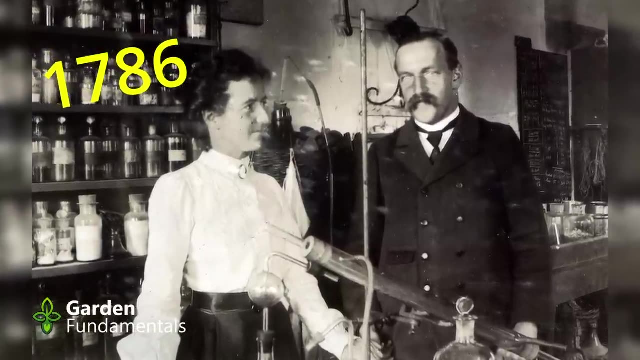 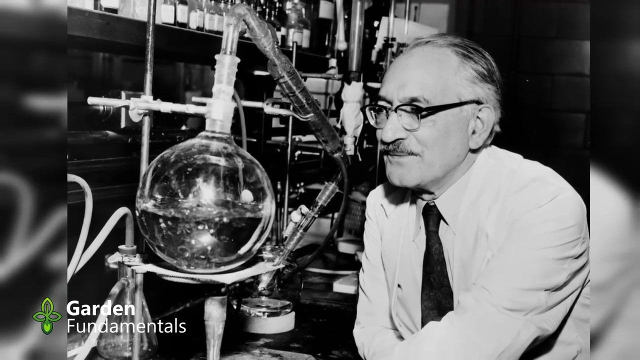 and humus. You can think of them as different types of humus. The first humus was extracted in 1786. That's a long time ago and it's been studied ever since. One of the early scientists working on this was Wakesman, who was one of the first to believe in the humus theory. But as he studied it, 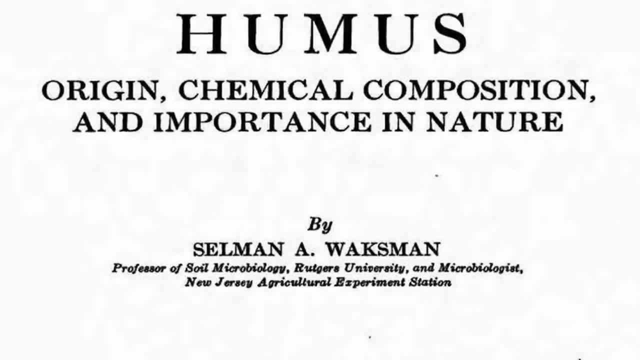 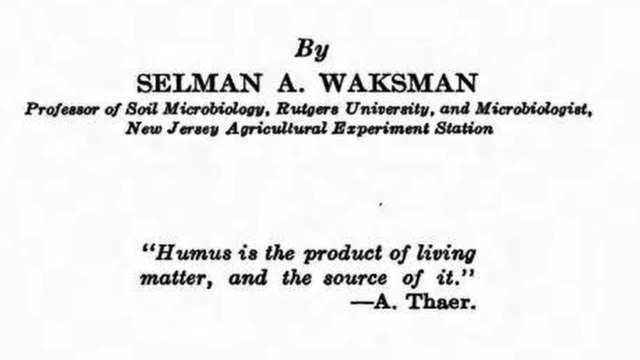 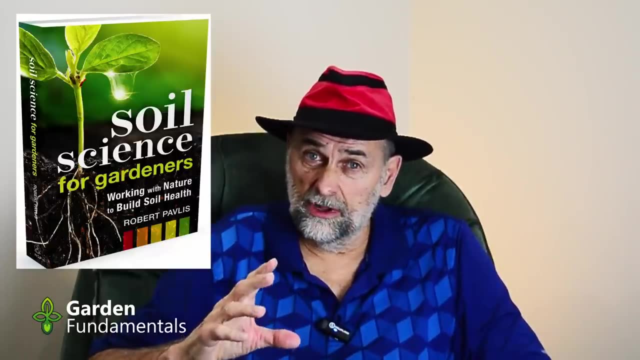 more. he changed his mind. In 1936, he published a book outlining the reasons why humus is so important. The idea of humus didn't make any sense. His views were mostly ignored by other soil scientists. But over the years someone would come along and say, geez, some of his ideas really. 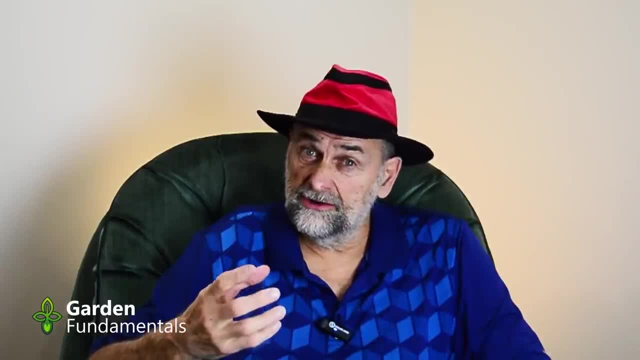 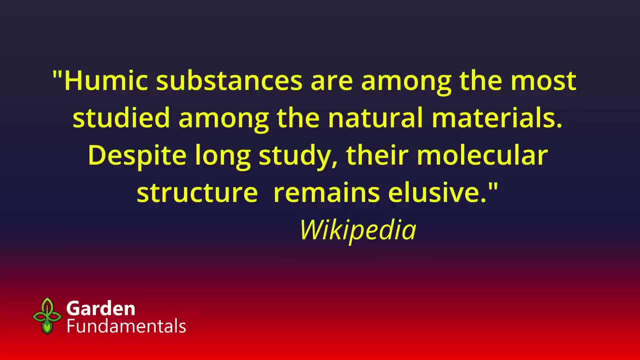 make sense. Maybe we should reevaluate our understanding of humus. What are these concerns? The first one has to do with the structure of humus. Here we have a very stable compound that makes up a significant amount of the organic matter. The humus is a very stable compound that. 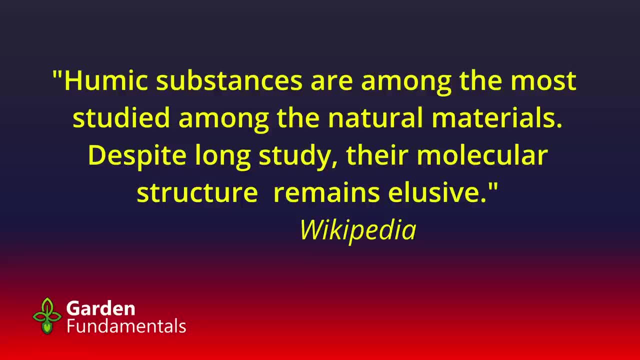 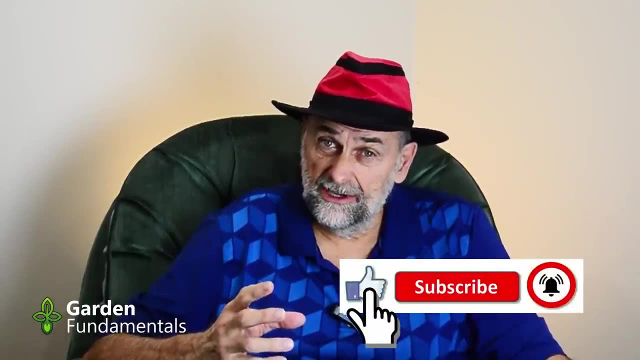 makes up a significant amount of the organic matter in soil, And yet over the last 200 years of studying this material, no one has been able to document its chemical structure. That is very odd, given the fact that hundreds of scientists have looked at humus and tried to define what it is. 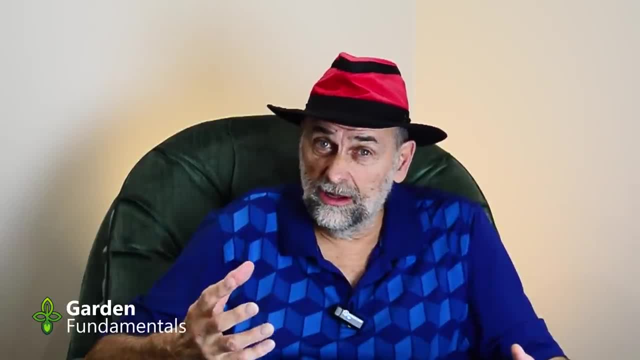 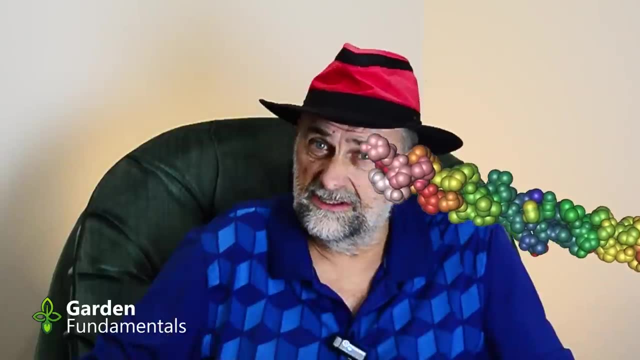 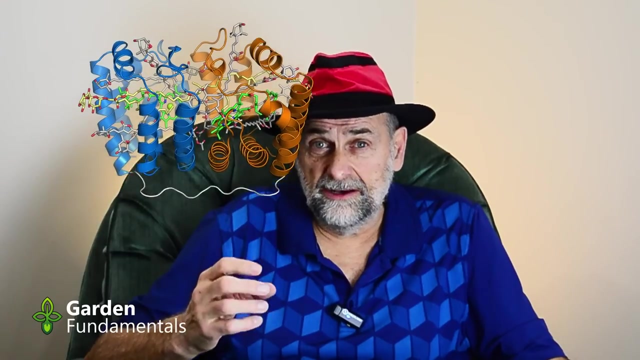 Now we're able to describe almost every large molecule we've found in nature and we know what the molecular structure of all these things are: Large proteins, DNA molecules, large polysaccharides. We can draw out their molecular structure and yet almost nothing is known about the molecular structure of humus. 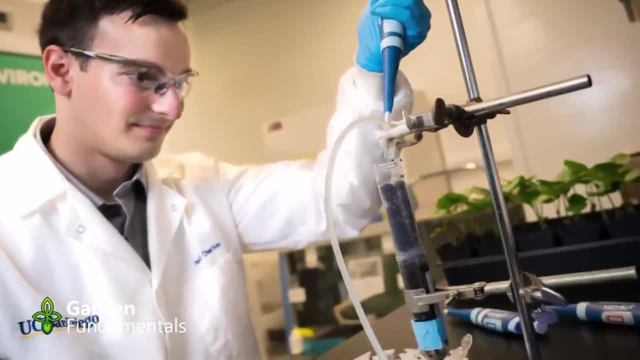 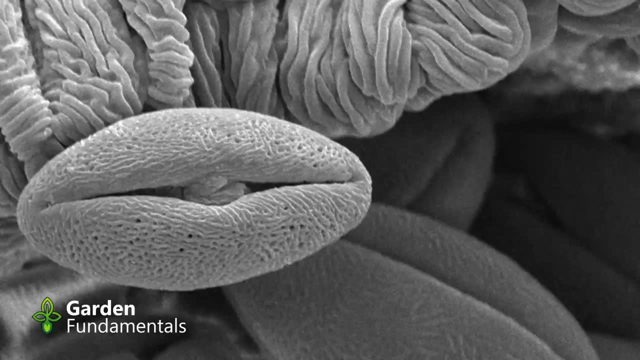 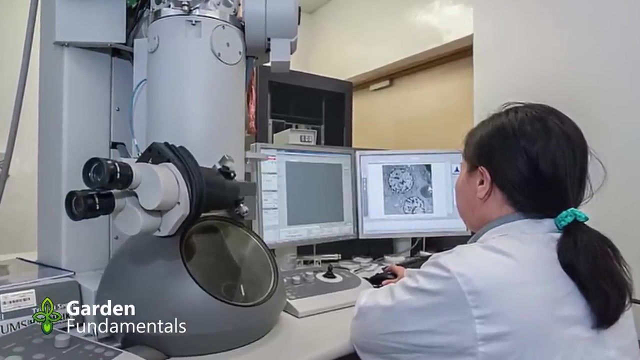 The second problem is just as mysterious: No one has ever seen humus in soil. Even with all of the modern-day equipment and all of the specialized electronic microscopes, we have no one has ever seen humus. Humus is only studied after it's extracted from soil, using very alkaline solutions. This is important because 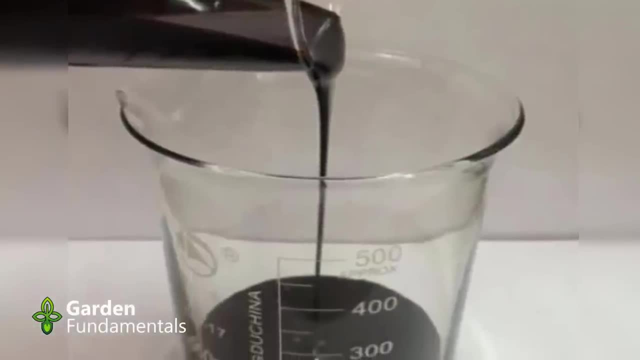 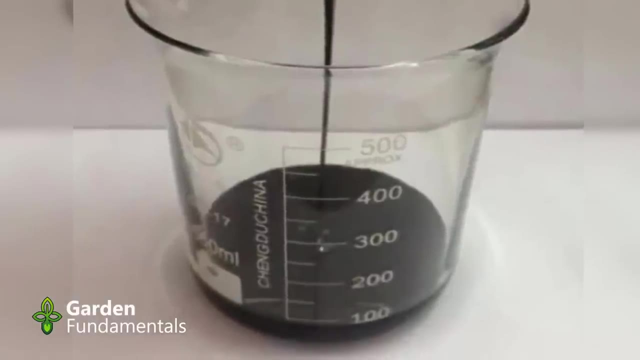 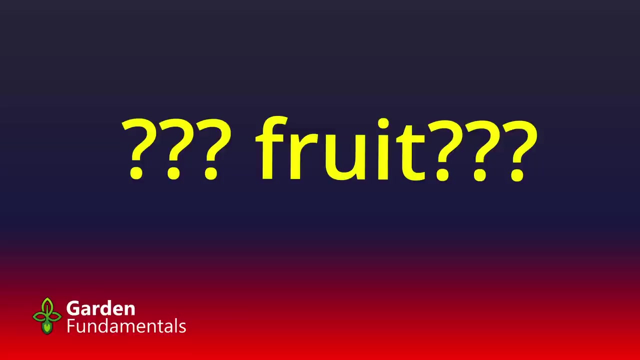 strong alkali solutions cause all kinds of chemical reactions, So by the time humus is extracted, it no longer looks the way it did in soil. Imagine trying to describe a new species of fruit that you've never seen before, and all you have are the feces from an animal. 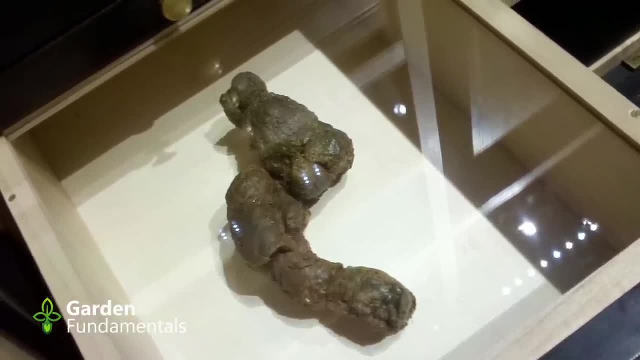 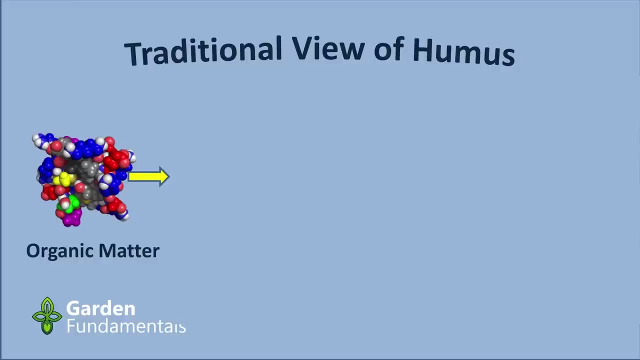 That is the challenge scientists have with humus: They can't actually see the material in soil. The third issue is an even bigger problem. Think back to that compost that is added to soil. It starts out as plant and microbe cells. These are slowly broken down into smaller and smaller pieces. 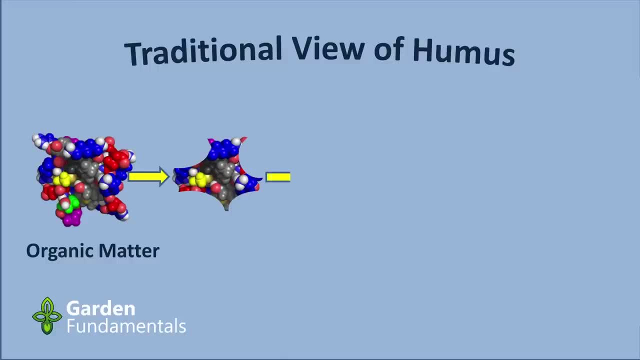 Cell walls are broken down to release some large protein, which are broken into peptides, which are broken down even more into amino acids And finally into nutrients like nitrate molecules. The same thing happens with all of the large molecules you start out with: They are slowly broken down into smaller and smaller molecules. 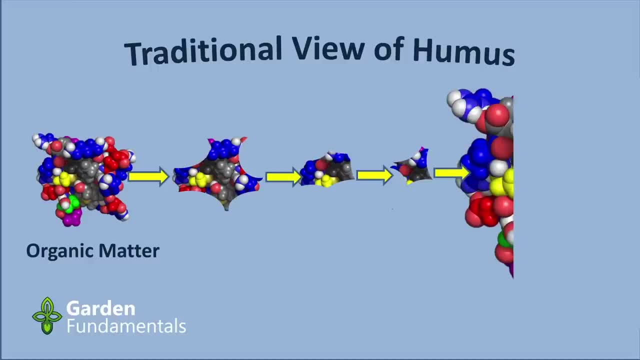 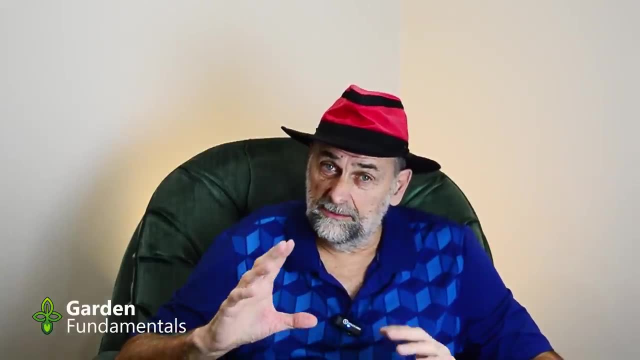 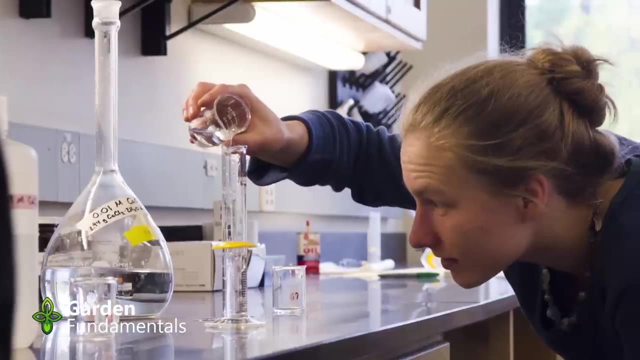 Then, at the end of this process, you suddenly have huge molecules called humus. How did that happen? No one in 200 years has been able to explain how we get smaller and smaller molecules and suddenly they're huge. Problem 4 has to do with the stability of humus. 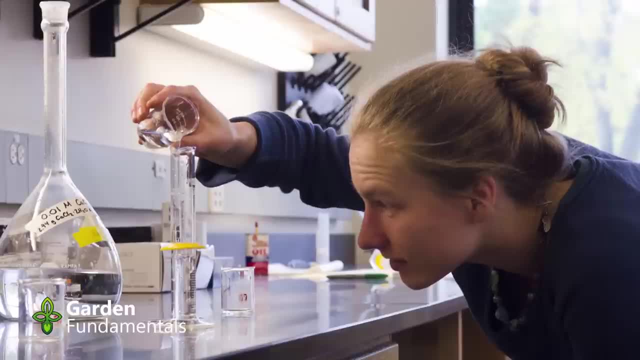 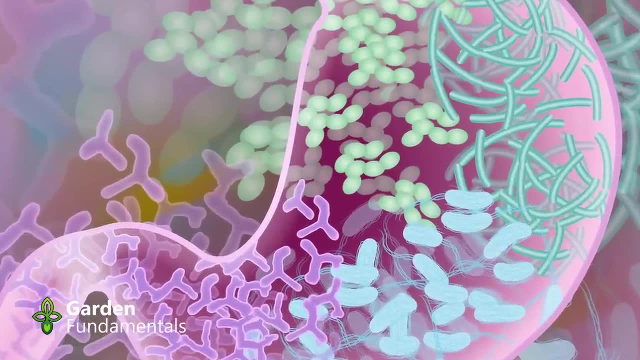 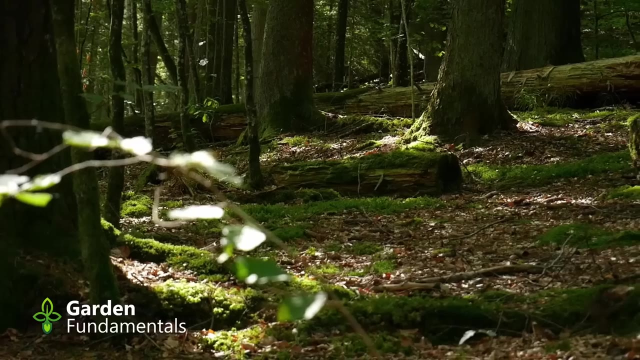 Every large organic molecule that exists in plants and animals can be digested by microbes, except for humus. Bacteria even digest rocks and oil, and yet humus is so stable it takes microbes hundreds or thousands of years to digest. How can that be? 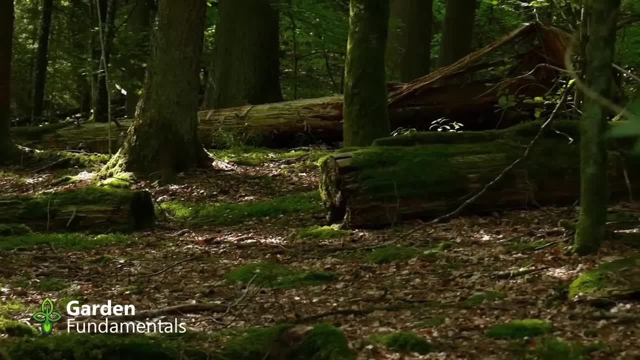 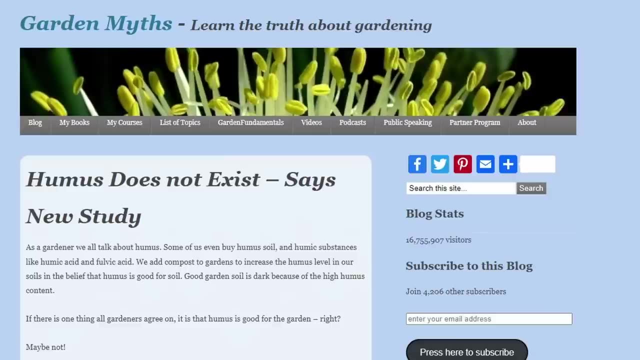 None of these four problems have been resolved And now more and more soil scientists are starting to believe the new theory about humus. Lehman and Kleber published an elegant description of this new explanation of humus in 2015.. You can read the details in my blog post, but the summary goes something like this: When organic matter is added to soil, microbes come along and digest it into smaller and smaller molecules. At some point, all of that original organic matter is completely digested. But where did it go? As the microbes digest the organic matter, they grow and they multiply. 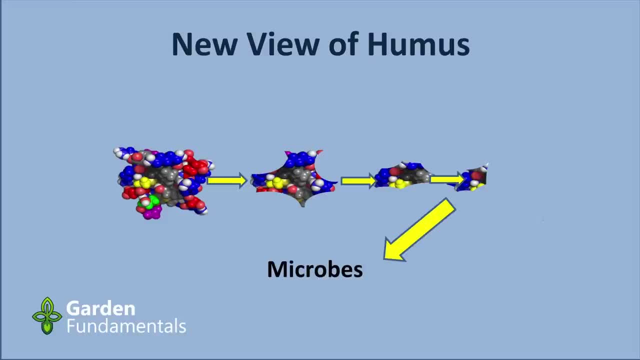 As they grow they take the nutrients and other small molecules and build them into large molecules inside of their own cells. That nitrate molecule that started as a banana peel becomes part of a new large protein molecule inside the microbe. When the microbe dies, its body is added to the pile of organic matter and the process starts all over again. 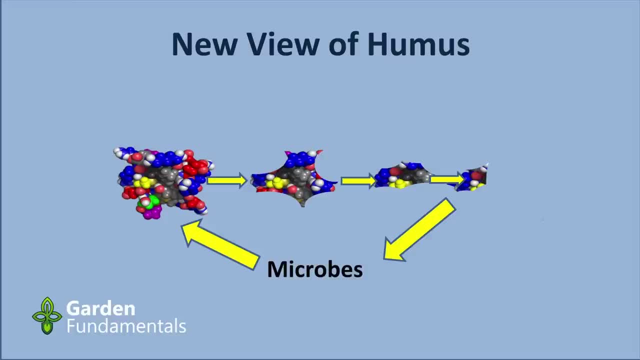 The cycle continues over and over again. Dead organic matter becomes small molecules, which are eaten by microbes, who turn them into large molecules, only to die and end up as fresh organic matter. This process does release carbon as CO2.. And the cycle would end unless there's a cure. 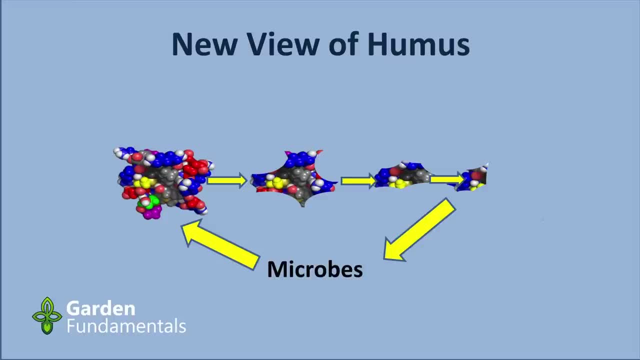 Unless there's a continual addition of new carbon, And that is where plants come in. They also use the nutrients to grow And at the same time they capture CO2 from the air. When they die or their leaves fall to the ground, they also become part of the starting organic material, adding new carbon. that keeps the cycle going. 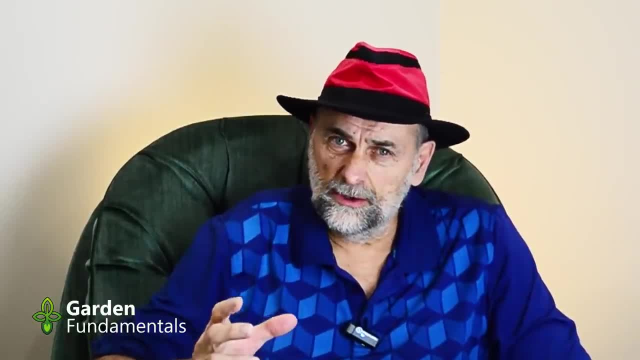 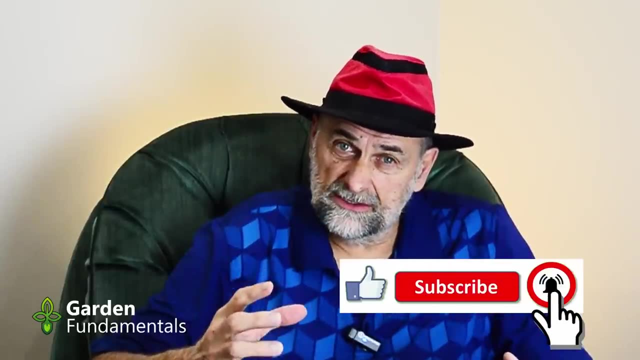 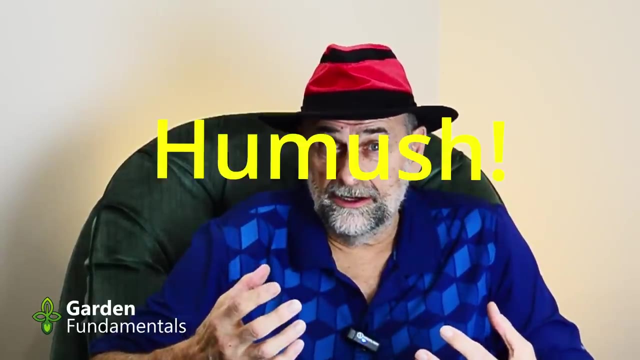 What about humus? There is no such thing in soil. When we apply an alkali solution to the soil, it takes all of the organic matter in that soil, both living and dead, and turns it into mush, Or as some people like to call it, humush. 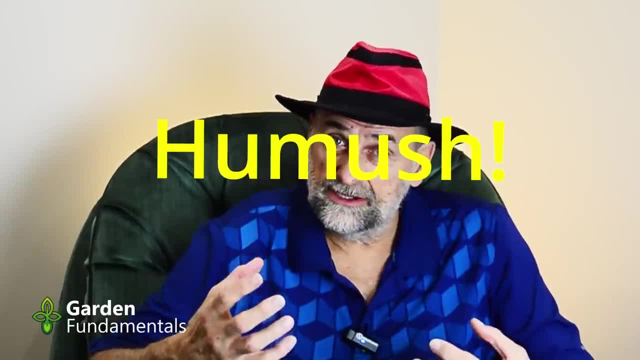 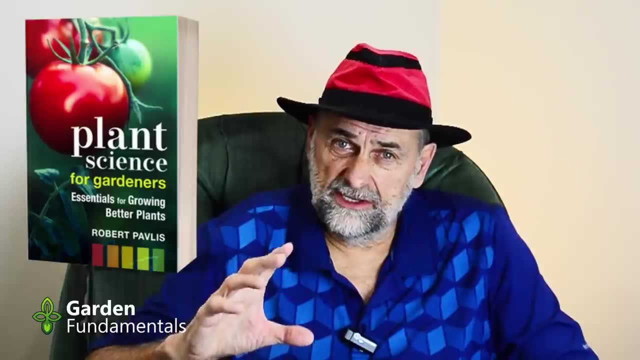 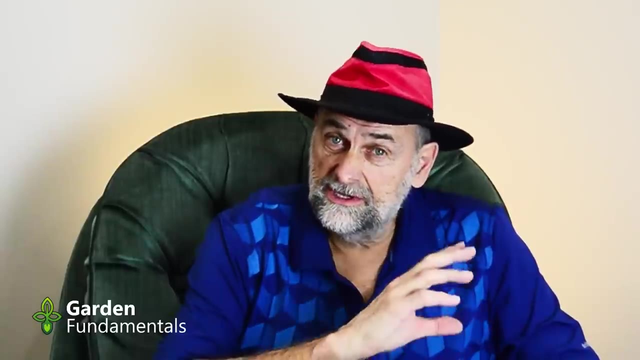 Humus is the artificial mush that's created when we treat organic matter in the soil with this strong alkali. Humus does exist in the lab as an extracted solution, but it never exists in the actual soil. What's in soil is organic matter, both living and dead. 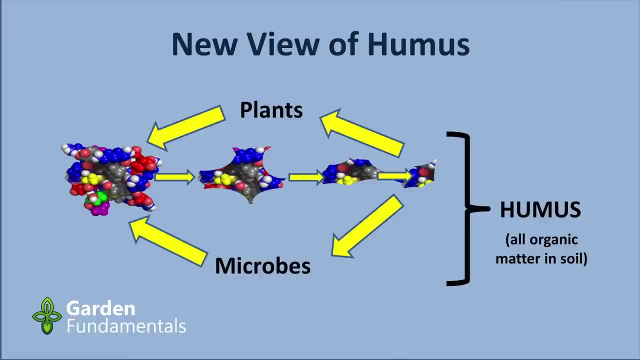 What does all this mean to gardeners? We should start thinking of humus as being the sum of all organic matter in soil, both living and dead. This does produce a healthy soil, largely because the cycling of molecules keeps a steady stream of nutrients flowing for plants. 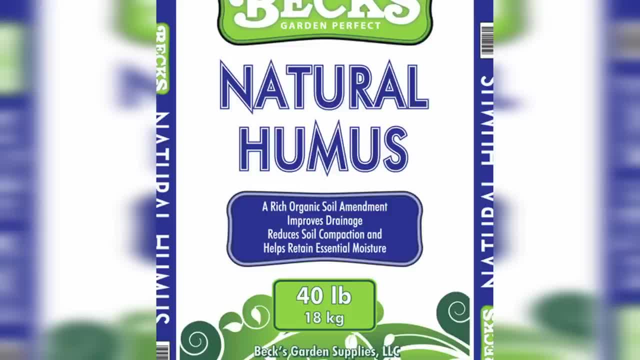 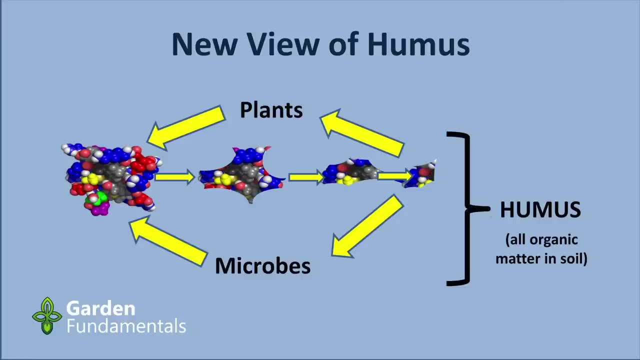 It means that you can't buy humus. Forget all the marketing nonsense about commercial plants. You can buy bags of humus If you want more humus. you simply add more organic matter to the soil. It also means that things like humic acid, fulvic acid and human do not exist in soil. 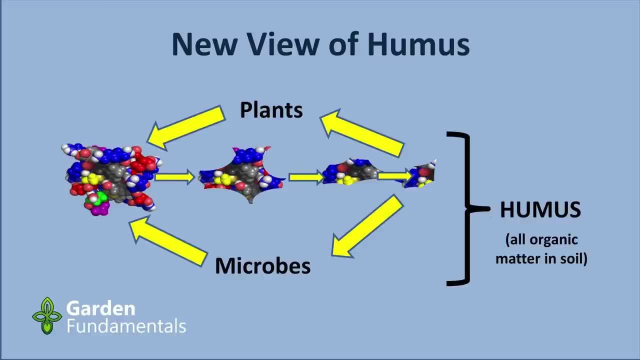 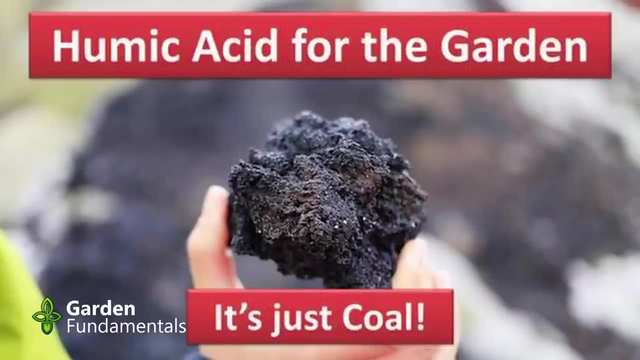 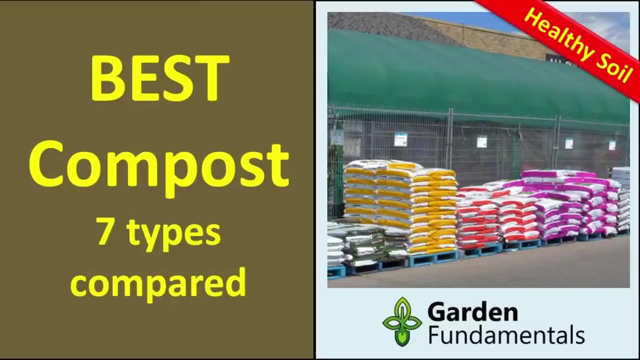 These are sold as commercial product, but now you know that these are a not natural in soil and b are not needed by soil. In fact, most commercial humic substances are made from coal. Why would you want to add this to your garden when compost and manure are much better options for adding organic matter?